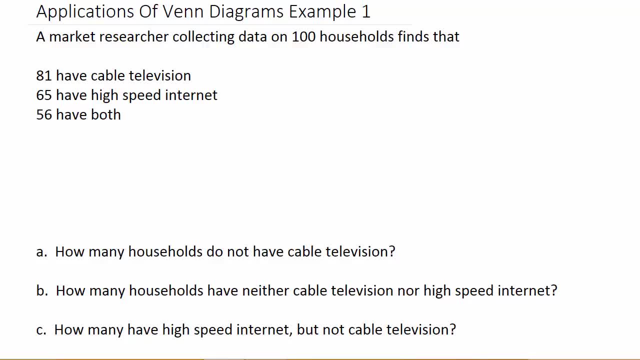 Alright. so here's an application for Venn diagrams. This one is going to have two sets: The people that have cable television and people that have high speed internet. I'll have another example- I'll put a link in the description- where there will be three sets So you can check that one out too. But I would watch this one because it will help you with the other one. It will help the other one make more sense. 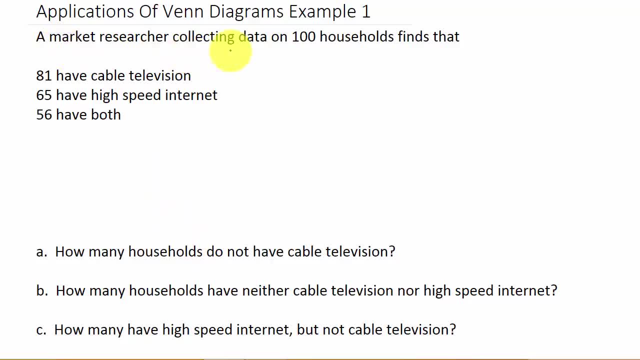 Alright, so let's get started. So it says. a market researcher collecting data on 100 households finds that 81 have cable television, 65 have high speed internet and 56 have both. Alright, so let's draw us a box here. 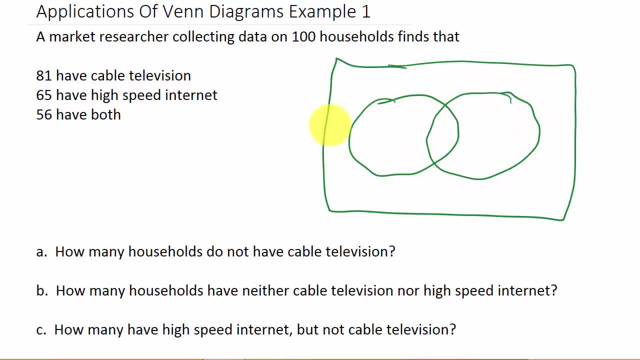 And we've got our two sets. So we'll call this one cable television, And we'll call this one cable television, And we'll call this one cable television And we'll call this one high speed internet. Alright, so let's get started. 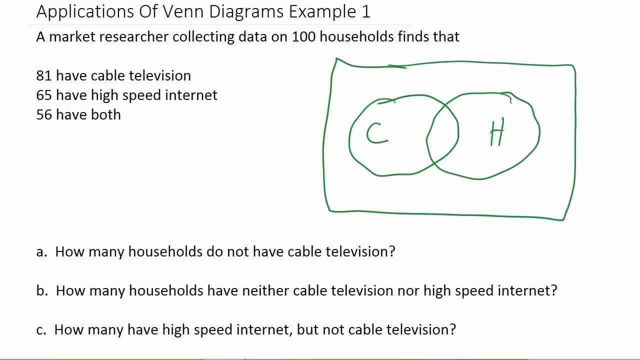 So here the best way to start is with what they have in common. So here it says 56 have both. Okay, so that's what they have in common. So that's where they're going to overlap. So well, where do they overlap? They overlap right here. 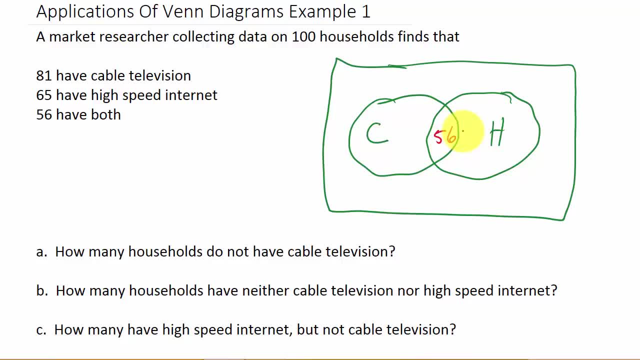 So this would be 56. Okay. And then it says that 81 have cable television. So 81 have cable television. So here we would have 25.. Now, how did I get the 25?? Well, 81 minus 56 is equal to. 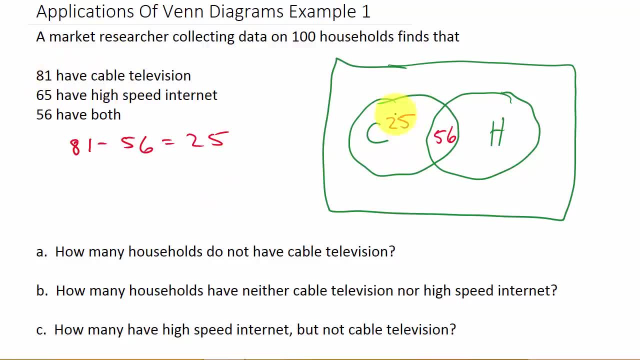 25.. Now keep in mind, the 81 does not go here. It says 81 have cable television. So these 25 plus these 56, that's 81. It just so happens that the 56 people here that have cable television, they also have. 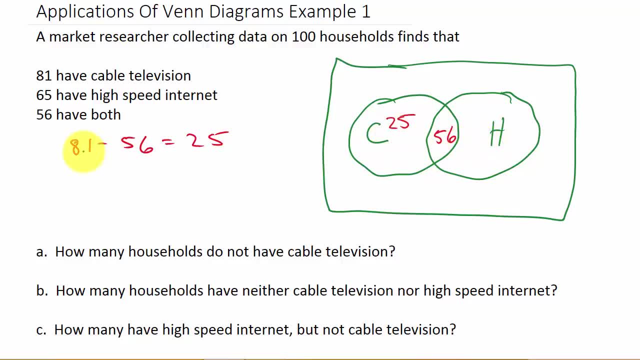 high speed internet. Now, the other reason that they have cable television is that they also have high speed internet. Now, the other reason that they have cable television is that they also have high speed internet. So this is the one that I knew that it was 81 minus 56 to get the ones that have cable. 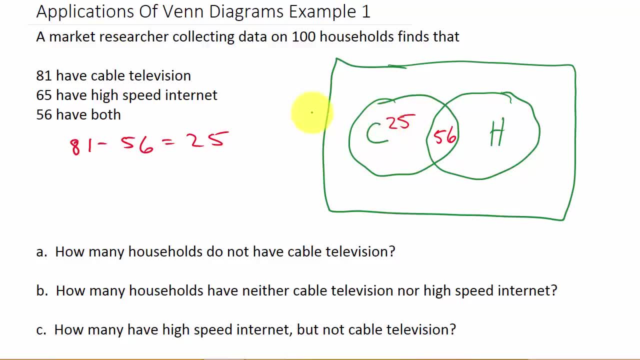 television here. Now how would I know if it would be 81 versus the 25 which I put? Well, if this would say 81 have cable television only then I would put 81 right here. But it just says 81.. 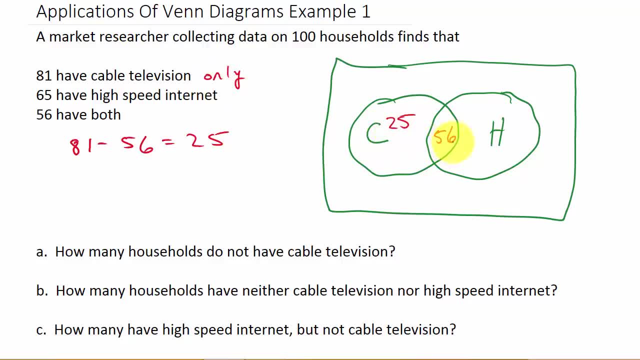 have cable television. so the 25 here plus the 56 here, that equals the total of the ones that have cable television. okay, it's just, of those 81 that have cable television, 56 also have high speed internet. all right, now let's look at this one. so it says 65 have high speed internet. so that means 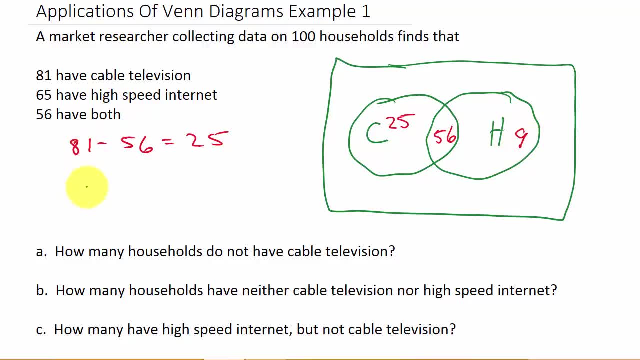 this would be nine. so how did I get that? well, 65 minus 56 equals nine, because it did. it did not say 65 have high speed internet only. okay, it just said 65 have high high speed internet. so it's the 56 here that have the Internet plus the nine here that have the internet totals the 65 that have. 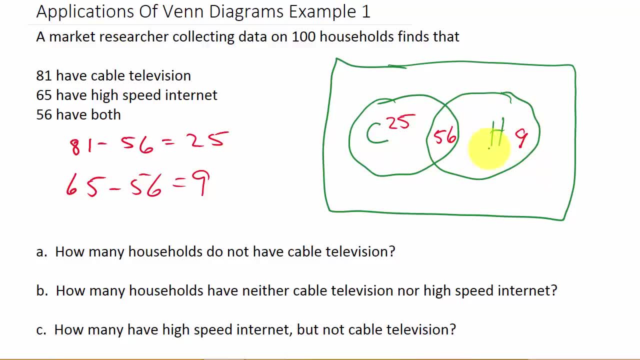 Internet. It's just, of the 65 that have internet, 56 of them also have cable television. All right, Now let's look at this out here. The people out here remember this is considered the universal set. That's everybody. 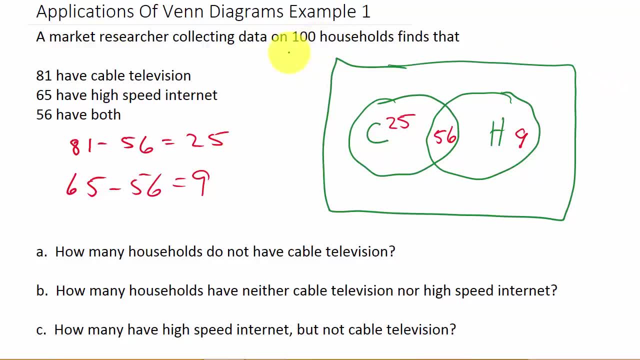 That's all 100 households, So that would be 10 out here. So how did I get that? Well, I know the whole thing. There's 100 households And if I subtract the 56 that have cable only, and I subtract, I'm sorry. 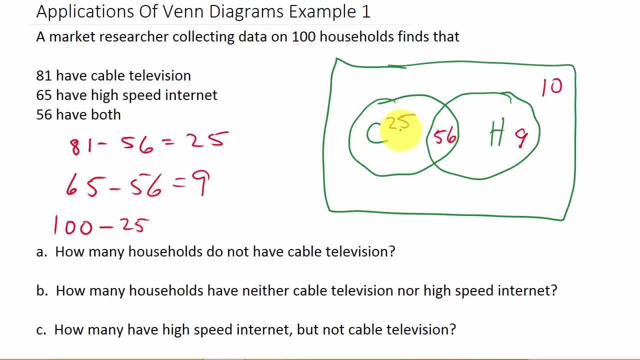 If I subtract the 25 that have cable only and the 56 that have cable and internet and subtract the 9 that have internet only, well, that equals 10.. So that means 10 of those 100 have neither one. 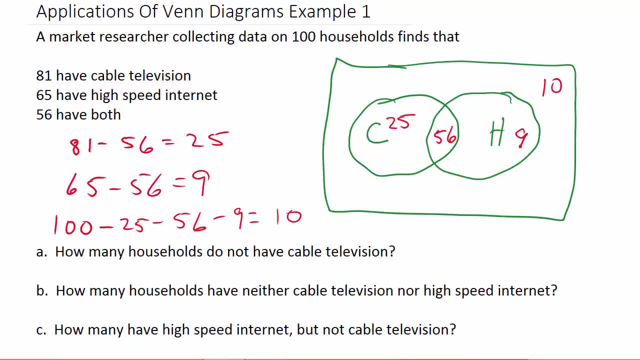 Okay, All right, So now we can go ahead and answer our questions. Once you get the Venn diagram filled out, the questions that it asks you are easy. So here it says how many households do not have cable television.